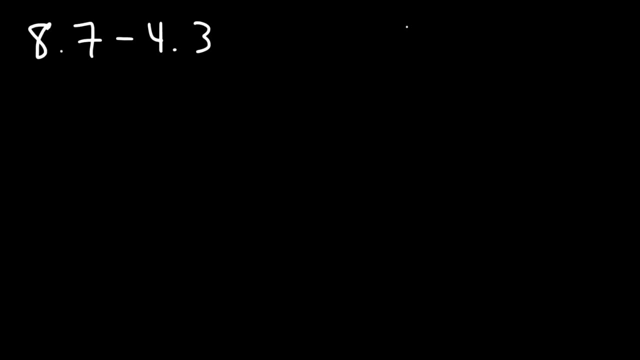 8.7 minus 4.3 and also 5.3 minus 2.8. So go ahead and work on those those two example problems. So let's start with the first one. So in the first 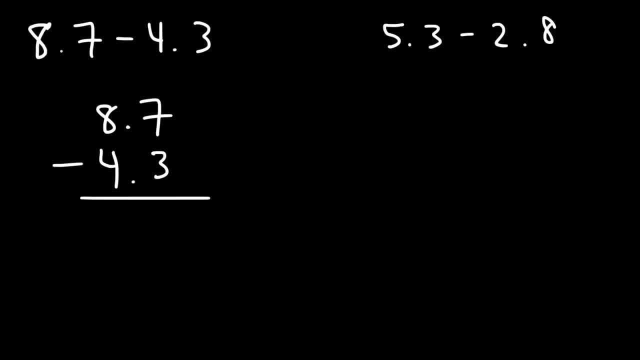 column we have 7 minus 3. 7 minus 3 is 4. Let's write the decimal point. And in the second column we have 8 minus 4. So the answer here is 4.4. 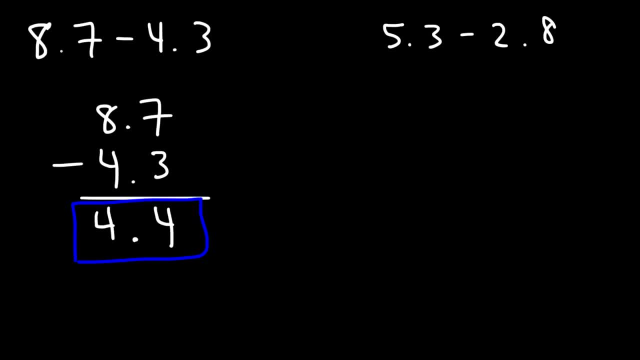 As you can see it's not that bad. Now the second problem is a little bit different than the first two ones. I mean this one and the one before that. Because we can't really do 3 minus 8. If we try to that's going to give us negative 5. And when you encounter a situation like this you need to borrow. Borrow a 1 from 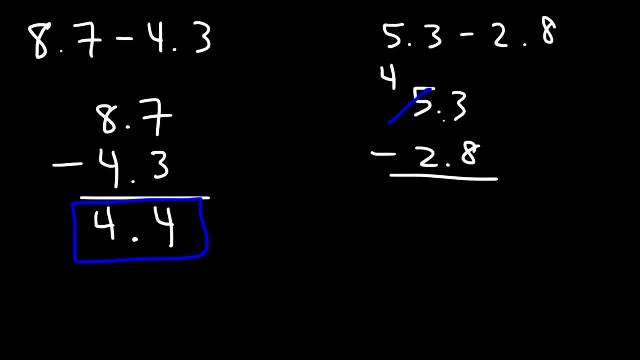 the 5. So the 5 becomes a 4. And you transfer the 1 to the 3. So the 3 becomes 13. 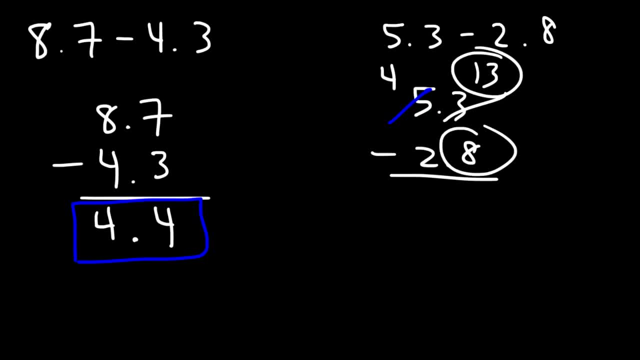 So now we can subtract 13 by 8. 13 minus 8 is 5. And then it's going to be 4 minus 2 which is 2. And so we have our answer 2.5. Now let's work on some harder 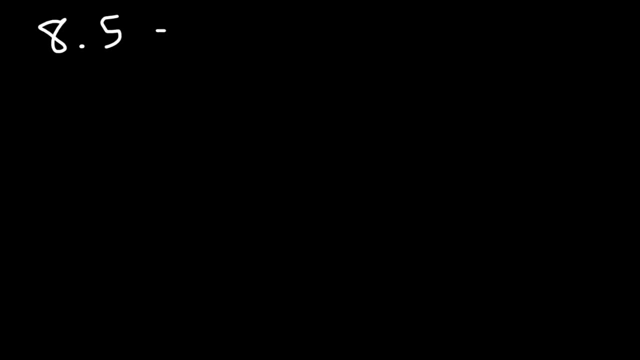 examples. So let's say we have 8.5. Let's subtract it by 6.23. So here we have a two-digit number. And here we have a three-digit number. So how can we line up these two numbers correctly? 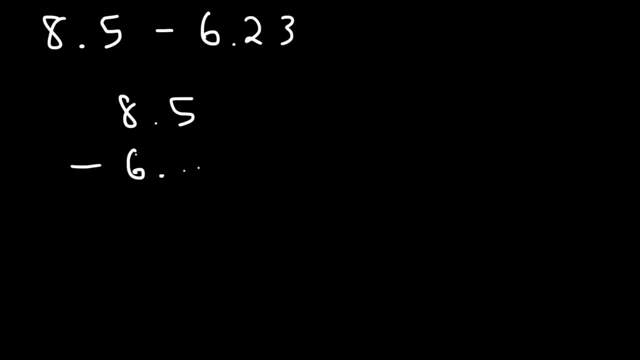 So remember when lining up the two numbers make sure that the decimal points are lined up correctly. Now to make it look better instead of writing 8.5 we can write 8.50. 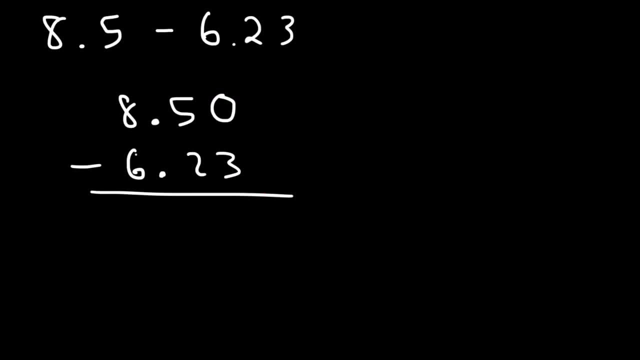 Now what is 0 minus 3? 0 minus 3 is a negative number. So we're going to have to borrow a 1 from the 5. So the 5 becomes a 4. And the 0 becomes a 10. So now we have 10 minus 3 which is 7. And then it's 4 minus 2, which is 2. And 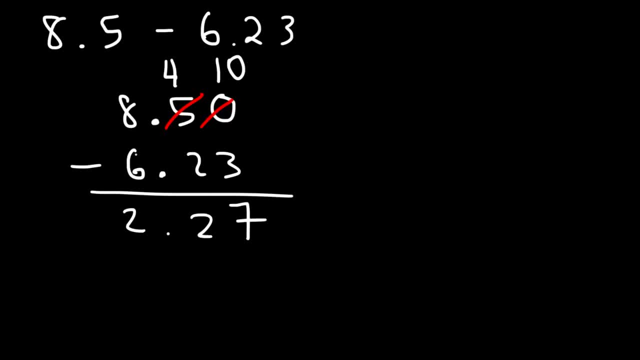 finally 8 minus 6 is 2. So the final answer for this example is 2.5. 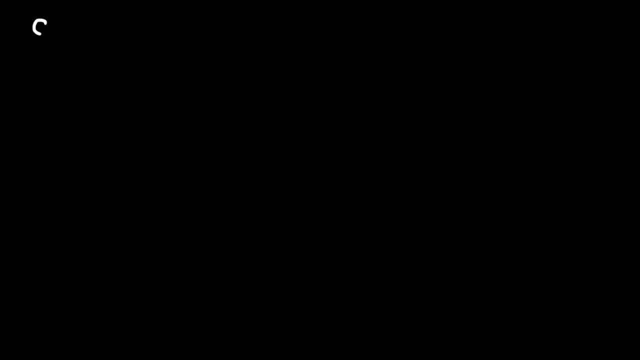 27. Now for the sake of practice, go ahead and try these two problems. 9.16 minus 4.17 and also 7.2 minus 5.83. So let's begin with this one. It's very similar to the last example. 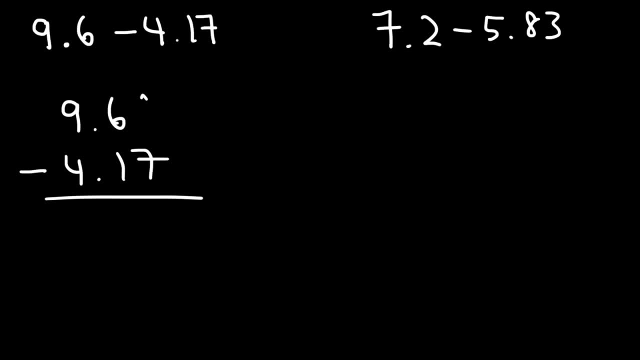 So let's line up the decimal points and let's add a 0 to 9.6. So we can't do 0 minus 7. So we're going to have to borrow a 1 from the 6, making it a 5, and transferring the 1 to the 0, which will make it 10. So now we can say 10 minus 7 is 3. And then 5 minus 1 is 4. 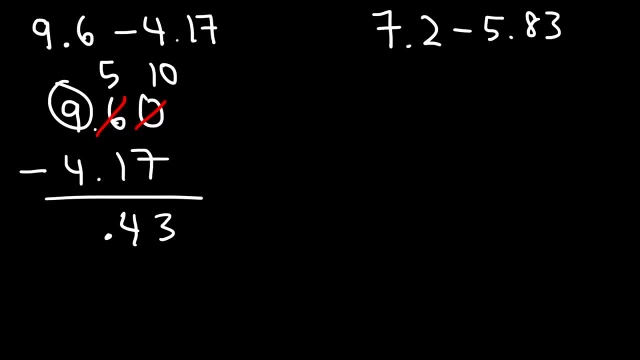 And 9 minus 4 is 3. I mean, no, that is not 3. 9 minus 4 is 5. 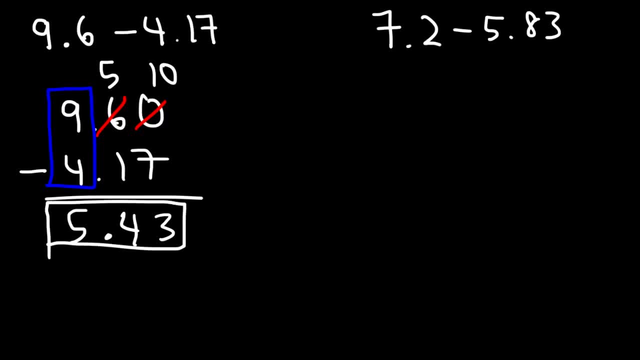 And so this is the first one. So let's do this one. So let's do this one. So let's do this one. This is the answer, 5.43. So let's do the same for this example. So let's begin by adding a 0. Once again, we're going to have to borrow a 1 from 2. So this is going to be 1. And a 0 is going to become a 10. So now let's subtract 10 by 3. So 10 minus 3 is 7. And then we can't do 1 minus 8. So we need to borrow a 1 from the 7, making that a 6, transferring the 1 to a 1 becomes 11. So 11 minus 8 is 3. And finally, for the last one, we have 6 minus 5, which is 1. 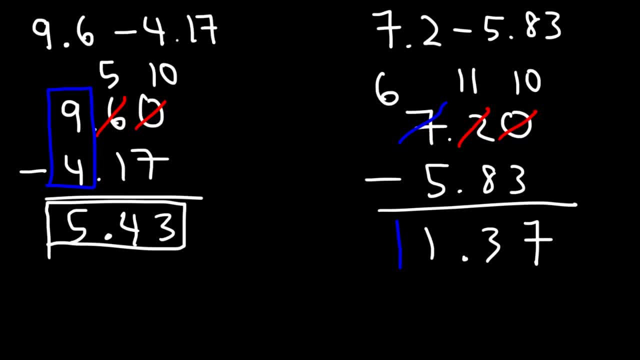 So the final answer for the third example in this series is 1.37. 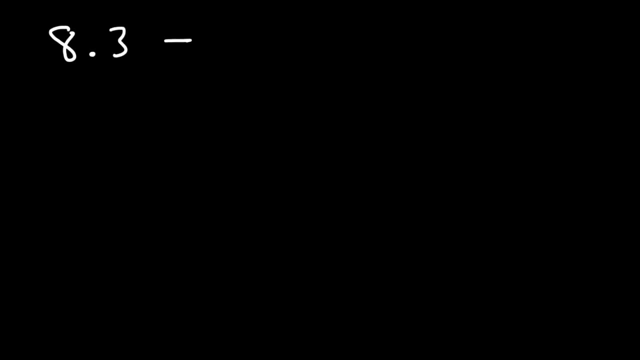 Now, what about subtracting a decimal number by a whole number? What result will we get here? The quick and simple method to subtract two numbers in this format is you could just subtract 8 by 5. 8 minus 5 is 3. And so the answer is going to be 3.3. Now, if you want to do it the safe way, you can simply line up the numbers. Now, instead of writing 5, we can write 5.3. And so we can do 3 minus 0, which is 3. And 8 minus 5, which is also 3. 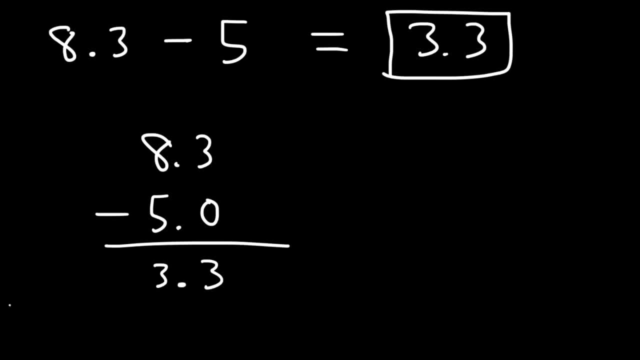 And so you can apply the same techniques to this type of situation. 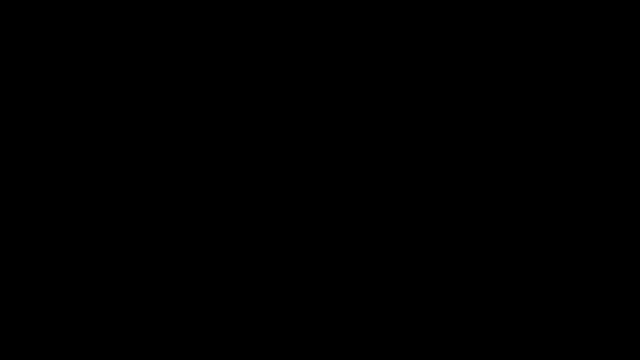 Now, instead of subtracting a decimal number by a whole number, let's subtract a whole number by a decimal number. So we can't just subtract 9 by 4 and say it's 5, because the 0.2 will decrease the 5 even further. Now, if you want to do it mentally in your head, you could do it this way. 9 minus 4 is 5, and then you have to say 5 minus 0.2, which is 4.8. That could work. But let's do it the old school way. 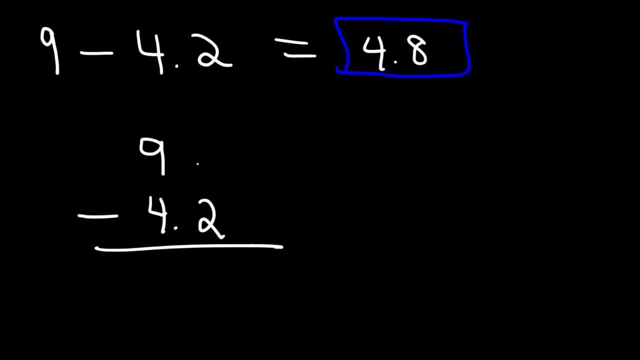 9 minus 4.2. So instead of writing 9, we need to write 9.0. Now, let's take away a 1 from a 9, making it 8. And let's transfer the 1 to the 0, changing it into a 10. So now, we can subtract 10 by 2, which will give us 8. And then 8 minus 4, which will give us 4. And so you get 4.8. Now, let's do it the old school way. Now, let's try another one like that. 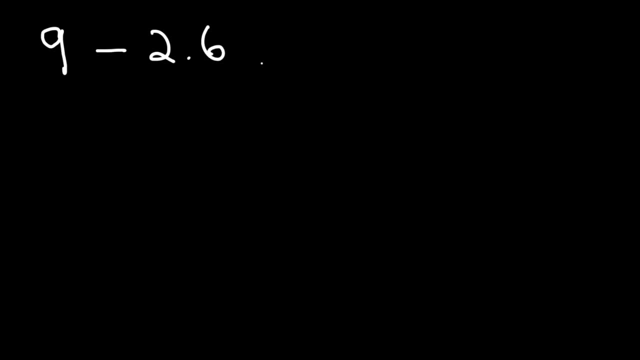 Let's do 9 minus 2.6. So what I'm going to do is, instead of writing 2.6, I'm going to break it down into 2 and 0.6, because 2 plus 0.6 is 2.6. 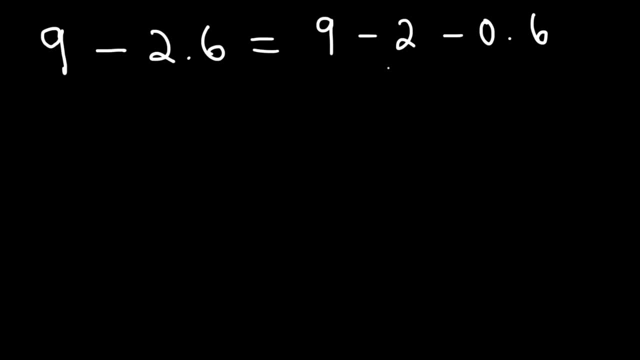 So negative 2 plus negative 0.6 is negative 2.6. 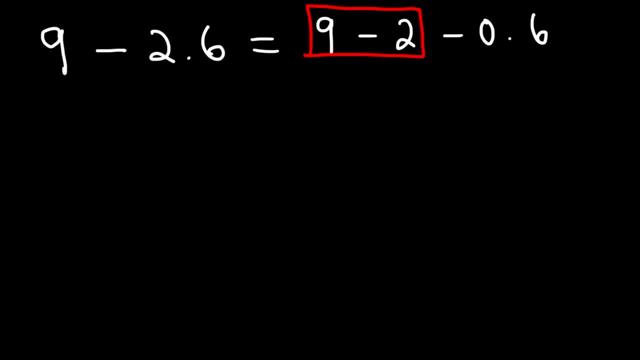 And so here, 9 minus 2 is 7. So I have 7 minus 0.6. And 7, you can write that as... 6 plus 1. So now, I'm going to subtract these two. 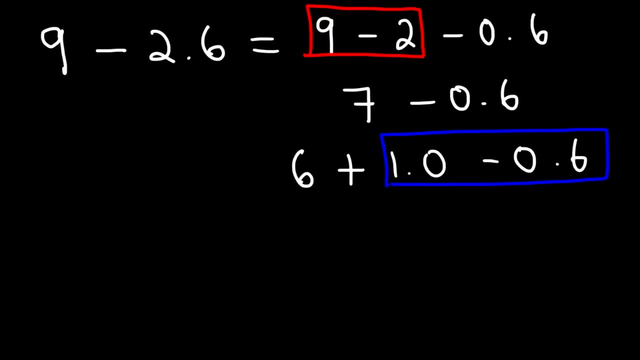 So 1 minus 0.6, if you think of 10 minus 6. 10 minus 6 is 4. So 1.0 minus 0.6 is 0.4. 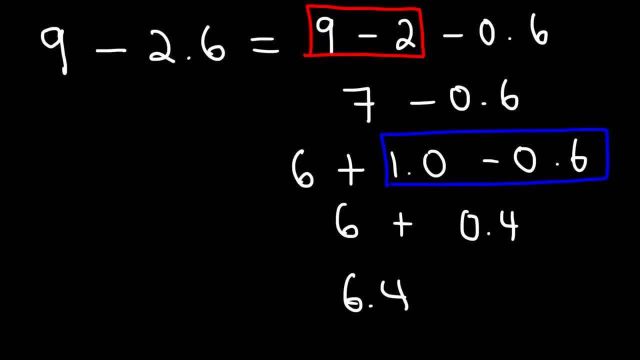 And thus, you have 6 plus 0.4, which is 6.4. And so that's another way in which you can do these types of problems. 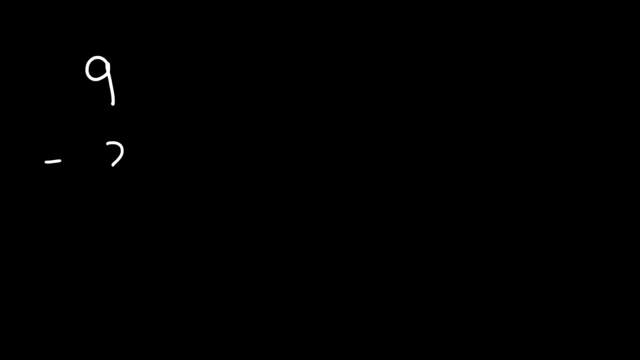 But now, let's confirm the answer. So let's do it. Let's do it this way. Let's add a 0. 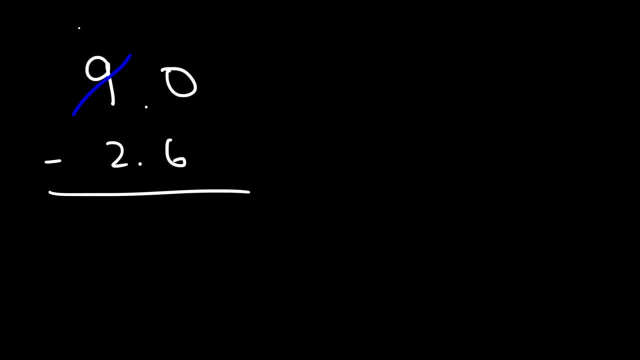 So first, let's take away a 1. Let's make this 8. And let's transfer the 1 to the 0, making that 10. And now we can subtract 10 minus 6, which is 4. And then 8 minus 2, which is 6. And so that will give us the same answer as 6.4. 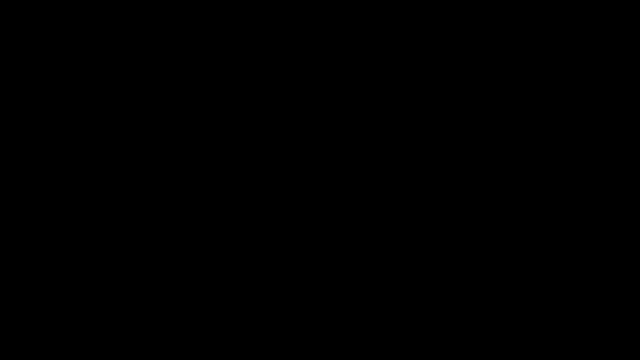 Now, let's work on a harder example. So let's subtract 7.5 by 4.368. So go ahead and try that. So all we need to do is add a few 0s. That's it. 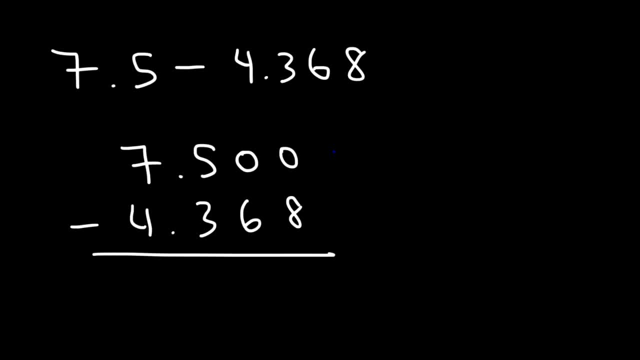 So first, let's borrow a 1 from this 0. So that becomes a 9, which means we need to borrow a 1 here. So that becomes a 4. And this changes into a 10. So 10 minus 8 is 2. And then after that, we have 9 minus 6, which is 3. And then 4 minus 3 is a 1. 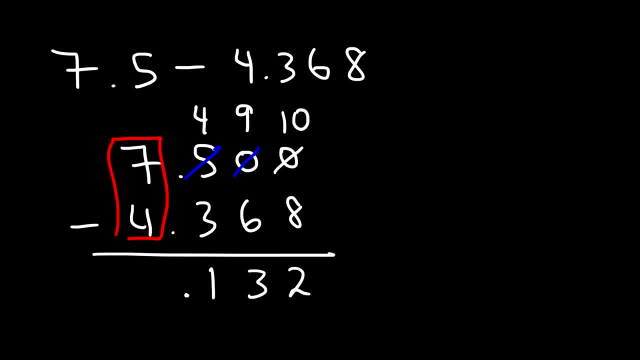 And for the last one, it's just 7 minus 4, which is 3. And so we get this answer. 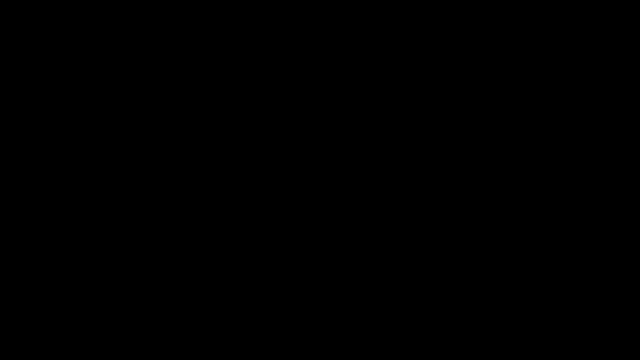 Now, what if we're doing a subtraction problem with three numbers, like this problem? 6.32 minus 3.451 minus 1.6. In a situation like this, I recommend subtracting two numbers at a time. So let's start with those two. So 6.32 minus 3.451. Let's add a 0. 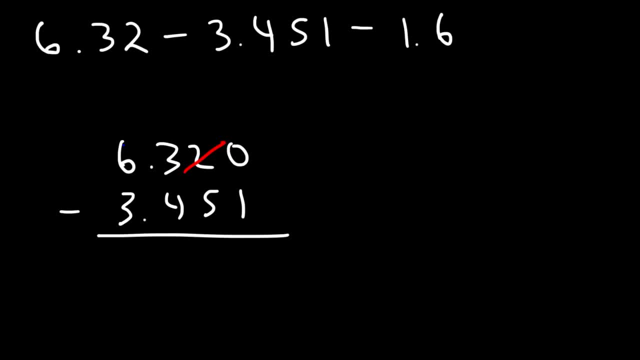 So we can't do 0 minus 1. So let's borrow a 1. Let's make this a 10. 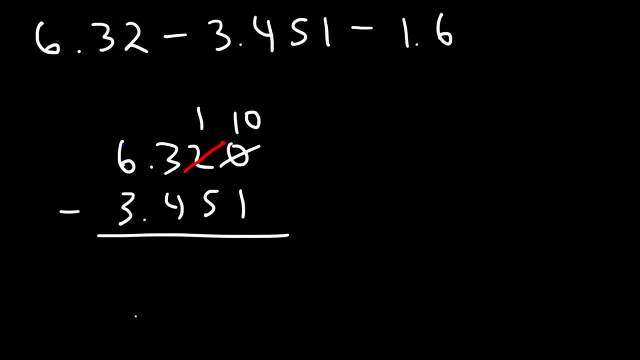 So 10 minus 1 will give us 9. And then we can't do 1 minus 5, because that's going to give us a negative number. 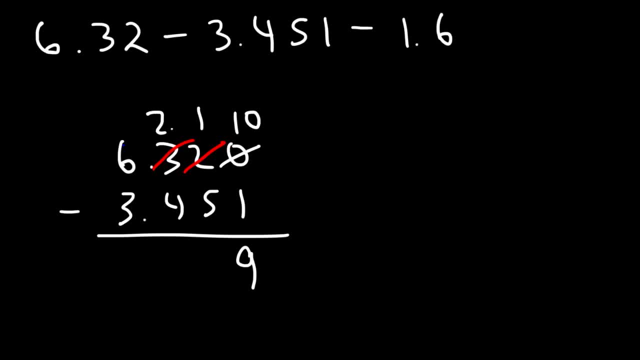 So let's borrow a 1 from the 3, making that a 2. And 1 becomes 11 on the right. So 1 minus 5 is 6. 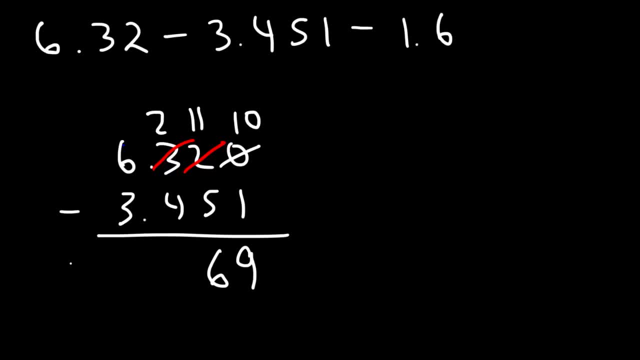 And we can't do 2 minus 4. So we need to borrow a 1 again, making a 6, a 5, changing a 2 to 12. 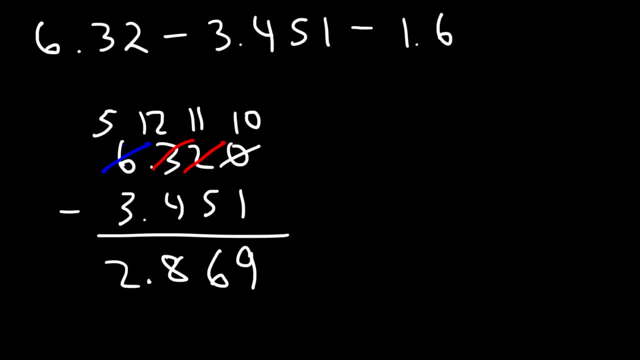 Now 12 minus 4 is 8, and 5 minus 3 is 2. 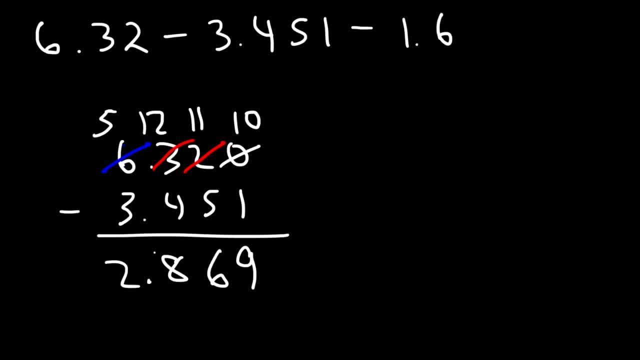 And if you have a calculator, you can just confirm it. And so 6.32 minus 3.451 is indeed 2.869. 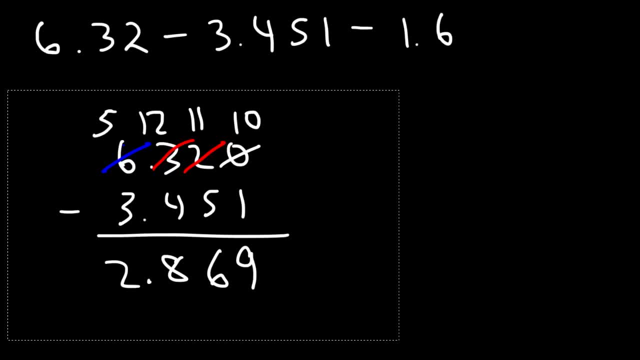 So now, let's replace the first two numbers with 2.869. And so let's subtract that by 1.6. 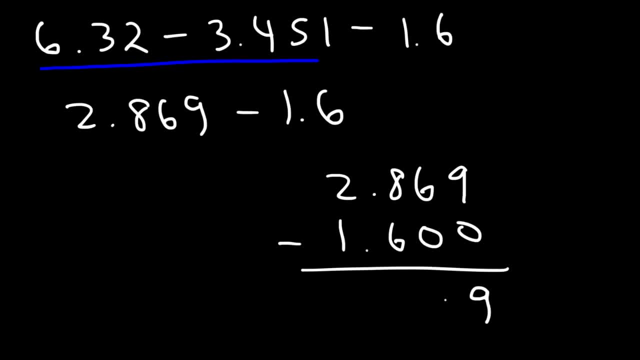 So 9 minus 0 is 9, 6 minus 0 is 6, 8 minus 6 is 2, 2 minus 1 is 1. 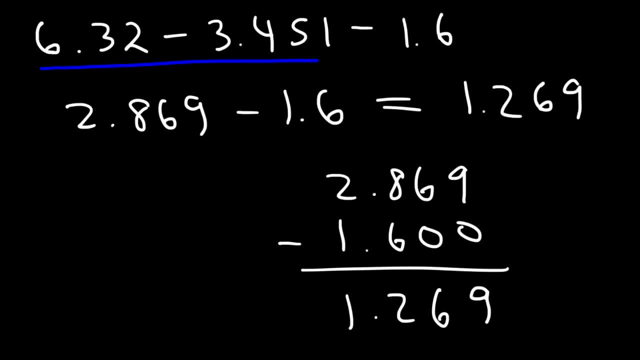 Thus, the final answer is 1.269. And so that's what you can do if you have a subtraction problem with three numbers. Thank you.